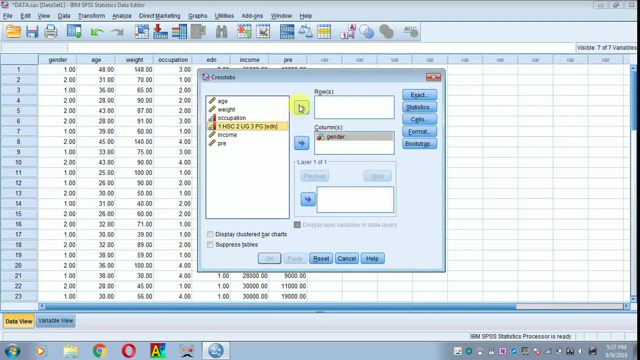 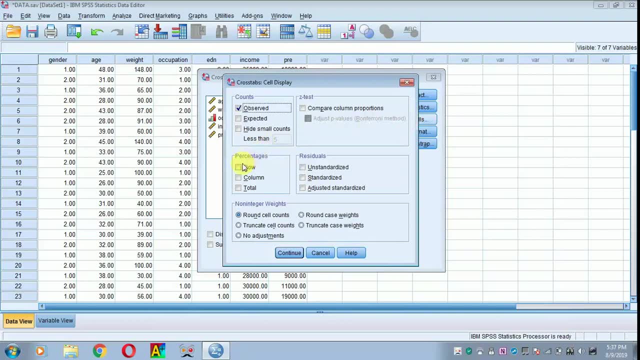 Here I am taking educational video. On the row side I am clicking cells over here. where you have got percentage You can click the column percentage or, if you want, you can click both row as well as total. Here I am going to click only the column percentage because mostly in the project or dissertation or thesis column percentage is mostly represented. 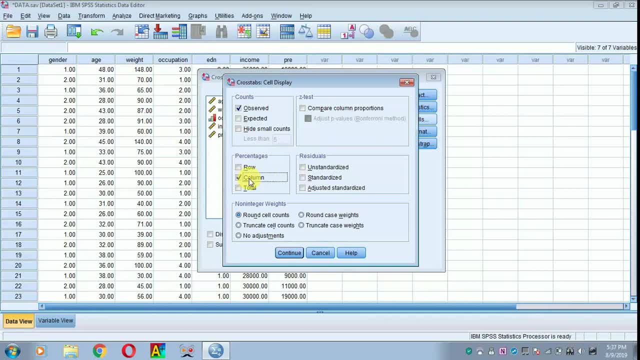 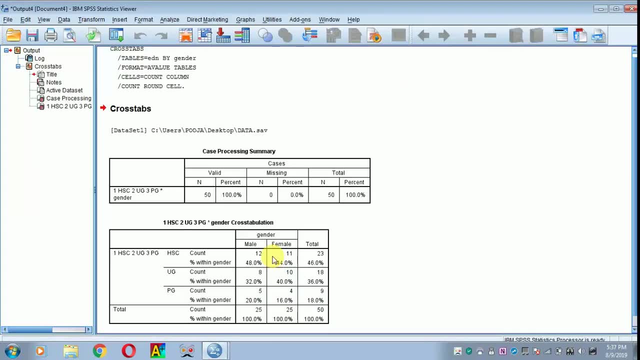 So that I have clicked column, Then click continue and then click ok. There you have got under higher secondary, how many are male and female and the respective percentage, Then the UG, the number of male, its percentage and female. Same way to PG also. 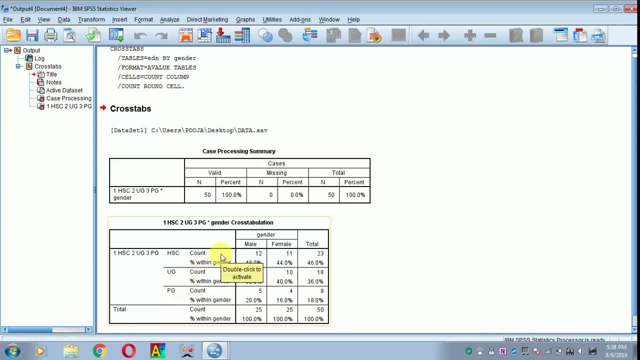 So this is how you have to find your column percentage for the variables. Thank you for listening.